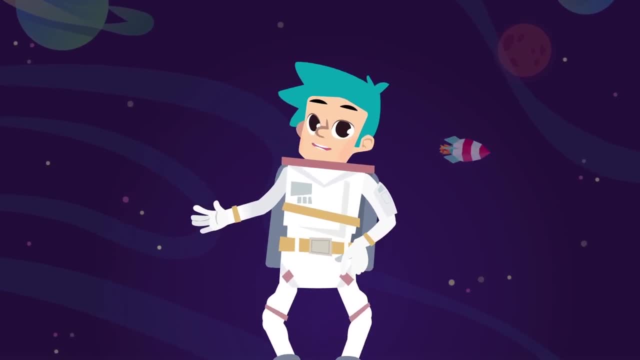 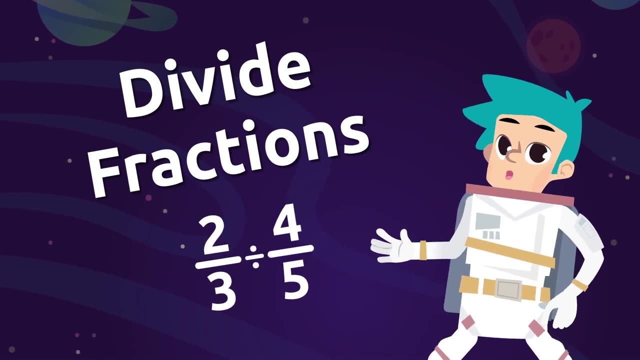 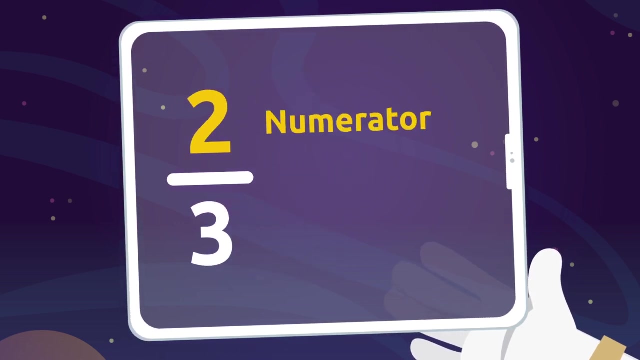 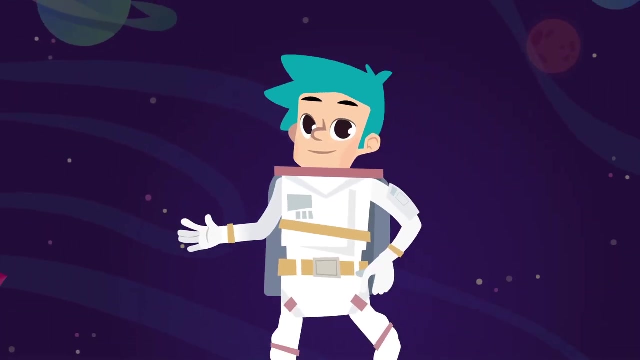 Hello again, friends, We continue practicing operations with fractions. Today we're going to learn how to divide fractions. First, let's recap quickly the parts of a fraction: The top number is the numerator and the bottom number is the denominator. Now we're ready to start. 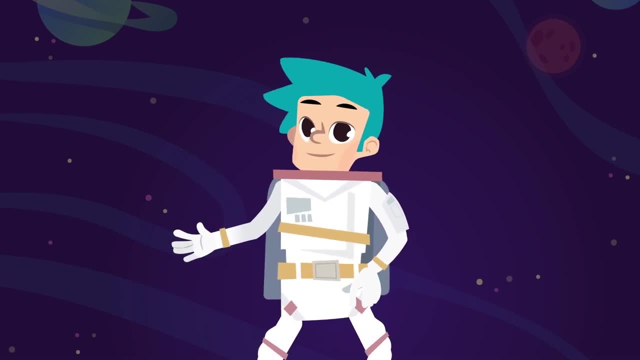 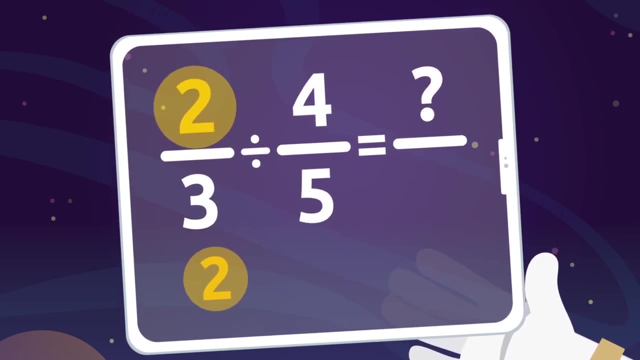 Dividing fractions is fun. Do you want to know how it's done When we divide fractions to find the numerator, we should multiply the numerator of the first fraction by the denominator of the second fraction. To find the denominator, we multiply the denominator of the first fraction by the numerator of. 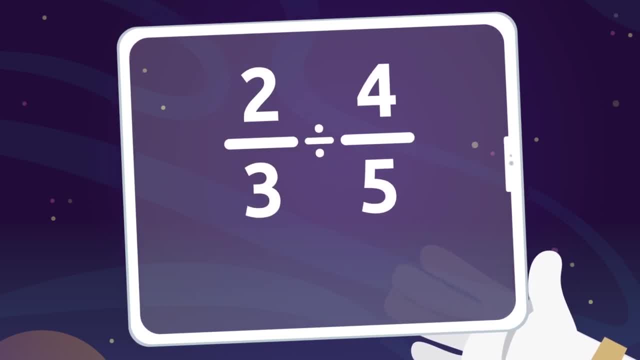 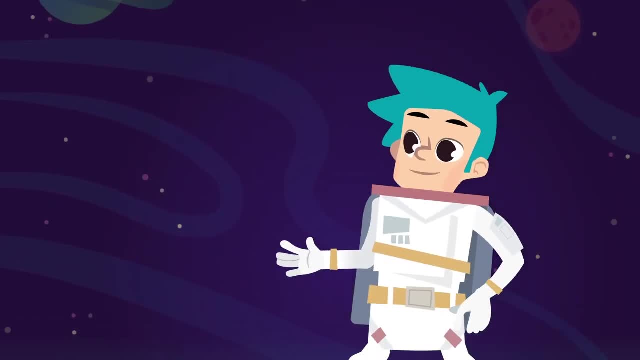 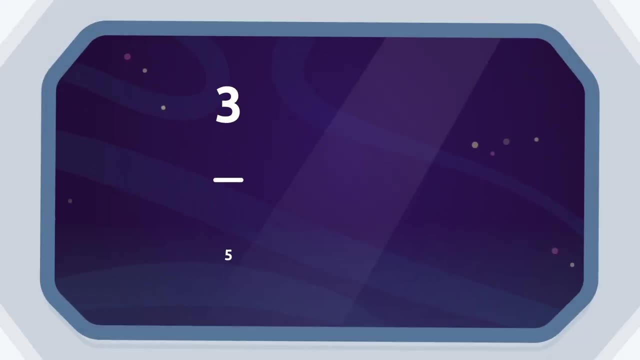 the second fraction. This means that to divide fractions, we cross-multiply them. Did you understand how it's done? Let's look at the next example. We need to divide three-fifths by one-half To find the numerator of the product we multiply. 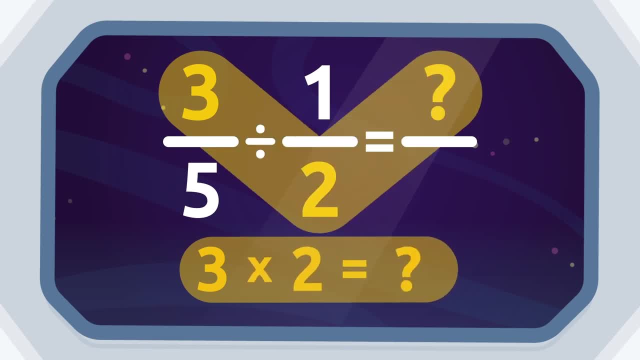 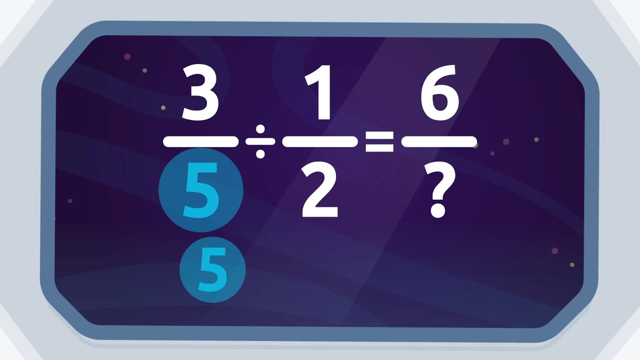 the numerator of the first fraction by the denominator of the second fraction, meaning three by two, which equals six. The numerator of the product is six. Now to find the denominator of the product, we multiply the denominator of the first fraction by the numerator of the second fraction, meaning five by one, which equals five. The denominator: 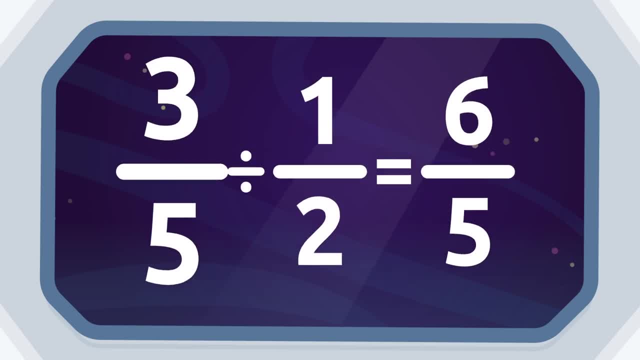 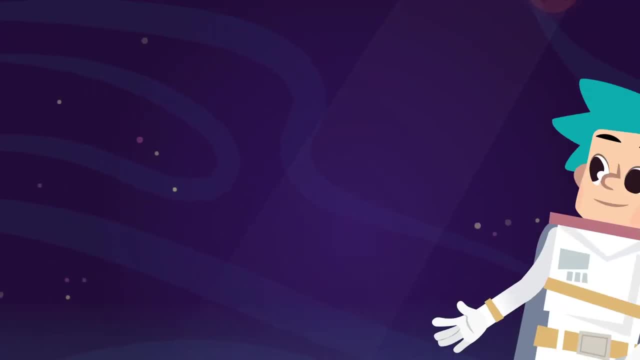 of the product is five. Dividing fractions is fun. Do you want to know how it's done? Let's look at the next example. divided by 1, half equals 6 fifths. Excellent, Let's look at the next example, Would you? 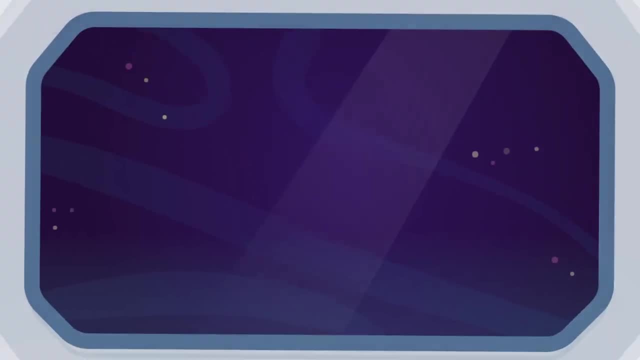 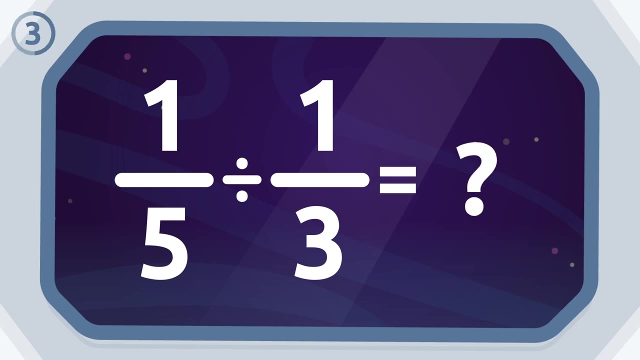 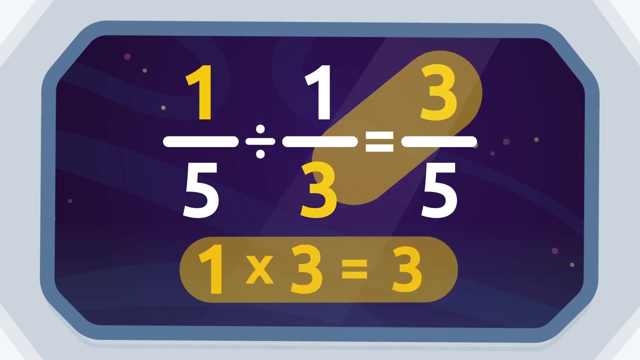 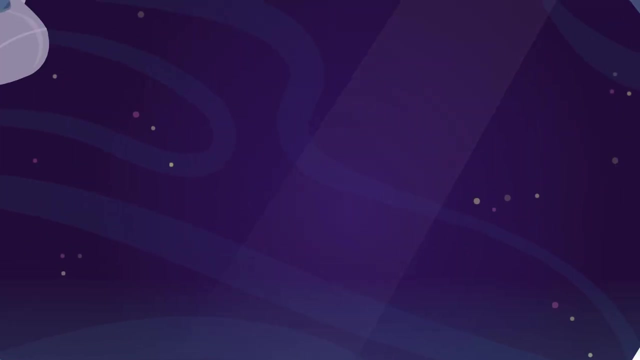 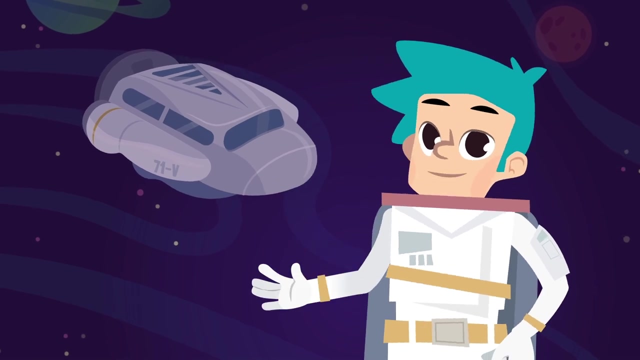 like to try doing this one yourself. 1 fifth divided by 1 third equals: Let's find out. if you got it right, 1 fifth divided by 1 third equals 3 fifths. Great job, Congratulations. Now you know how to divide fractions. You're a real expert. See you on the next video.